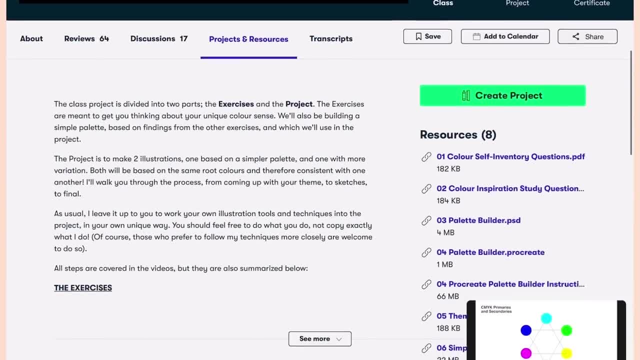 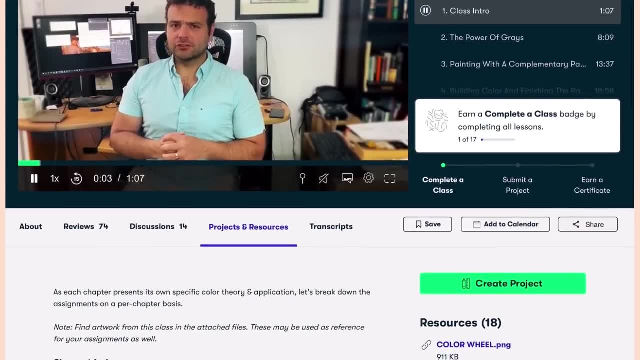 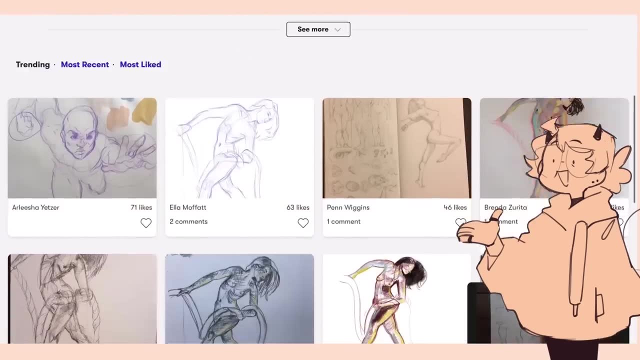 One Palette: Illustrator, Discover How Colour Works in Your Art by Tom Forrest, to the Colour Survival Guide by Marco Busi. Both these classes offer a unique perspective to the use of colours. There are so many more classes touching on this subject too, with unique perspectives and insight, Not just on the creative and physical side of learning. 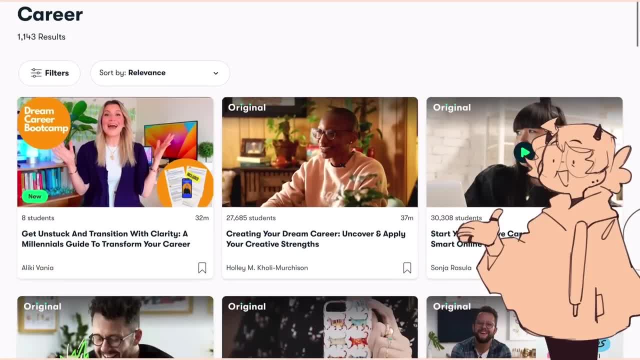 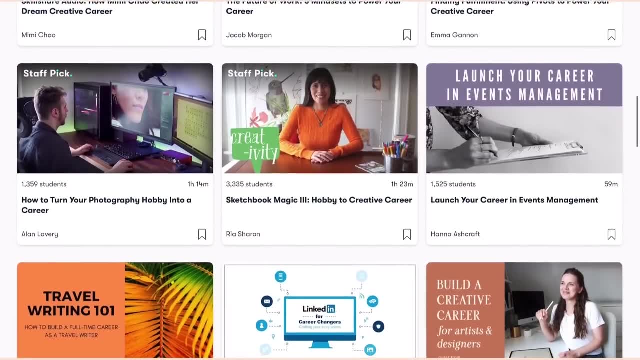 Skillshare also offers classes on developing and choosing career paths, from working in the creative field to managing finances. They have many more classes to further your career and help reach your goals. It's always fun to learn new and interesting things, whether that just be for fun. 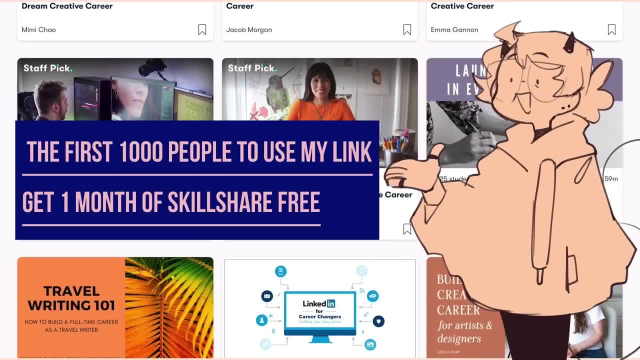 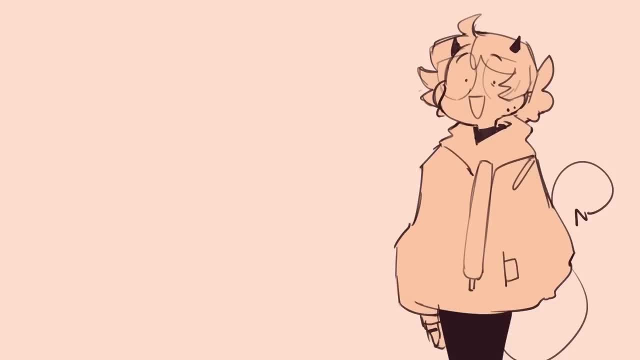 and hobbies or to build a career. Skillshare is offering one month free to the first 1000 people to use the link in my description. Thank you again for the support, Skillshare. and now on to the video. I hope to split today's video into two parts: one where I cover colour theory. 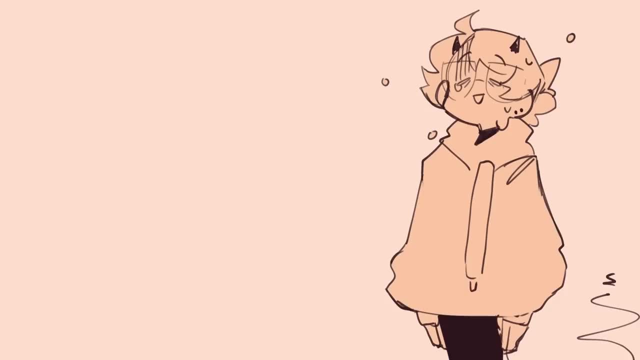 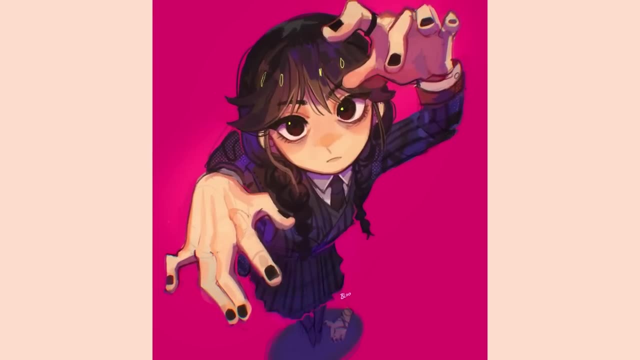 and the other where I show how I pick colours using colour theory. So, basically, colour theory is a collection of rules and guidelines that artists use to communicate to the viewers How well colours go together, can affect the atmosphere of the world and how they affect the world as a whole. So if you want to learn more, 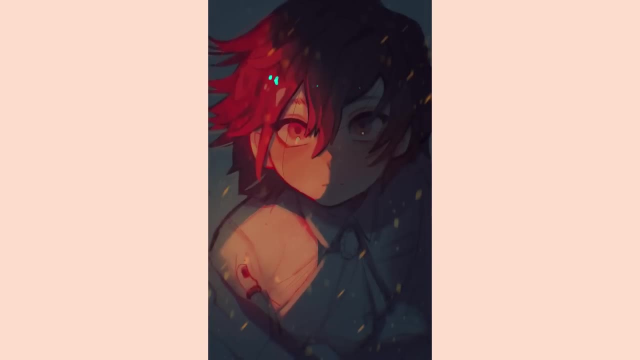 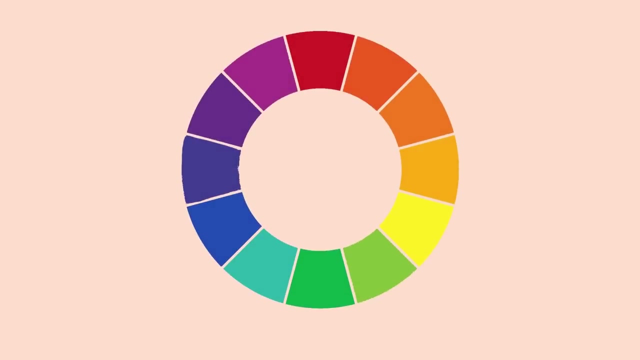 the colours can be used to guide the viewer's eyes to what is important in the piece, to show emotions or create a feeling or atmosphere. Now, the colour wheel is the basis of colour theory. It is made in the thought of the relationships between colours and how they affect each other. Here's what the colour wheel looks. 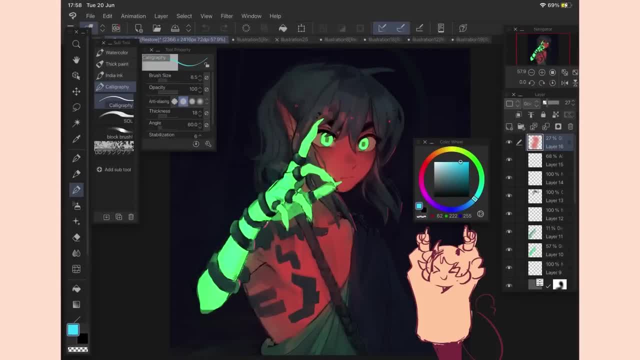 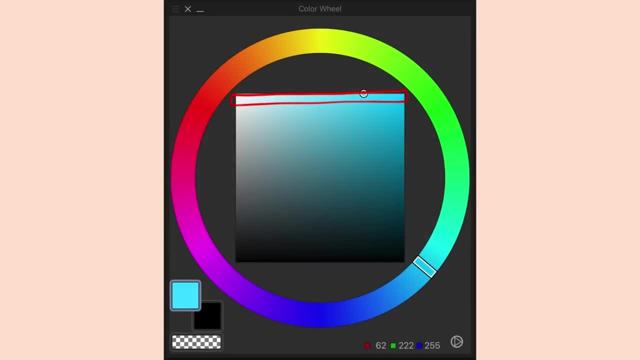 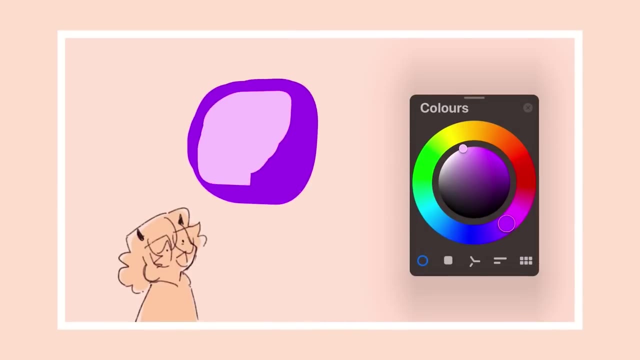 like It can be found in most digital art programs. The outer circle is called the hue. This is where you can find and select different colours. This section over here is the saturation. Saturation is the intensity of a colour. Here I have a very saturated purple, but I can desaturate it and 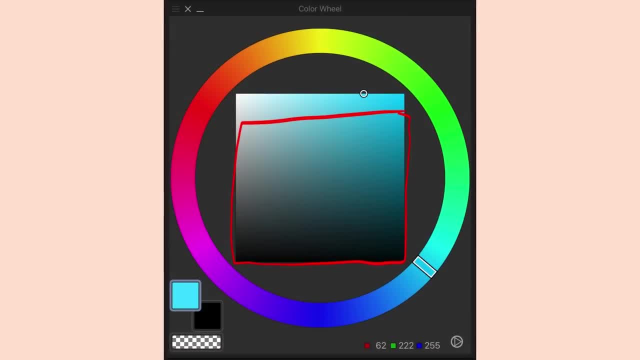 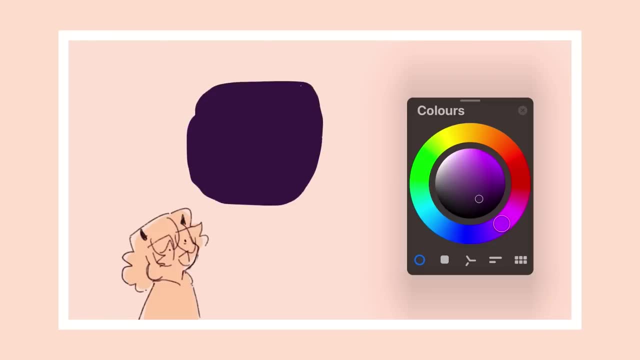 make it look lighter. The value is the brightness or darkness of the colour. You can change the value of the colour by adding more black to it or selecting this part of the colour wheel. So like this: Now this purple looks a lot muddier because I have changed the value by adding more black to. 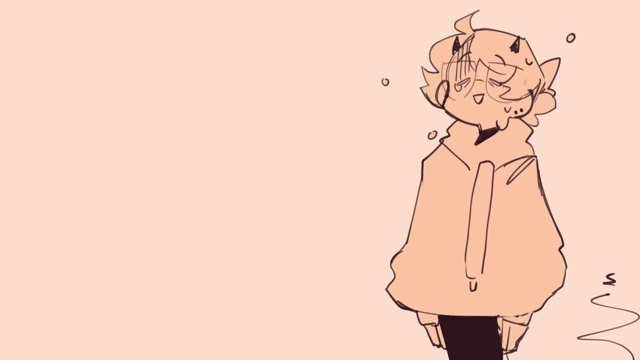 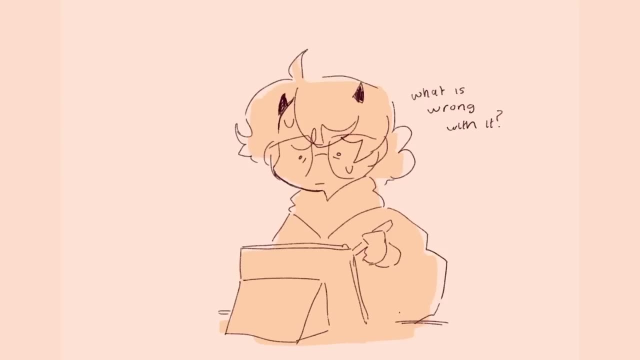 it Now. I feel like there's so much more I can explain about values, but I would keep that for a full video in the future. For now, just the basics is good. Colour saturation is actually the biggest culprit to colour picking. Highly saturated colours can make a piece restless. 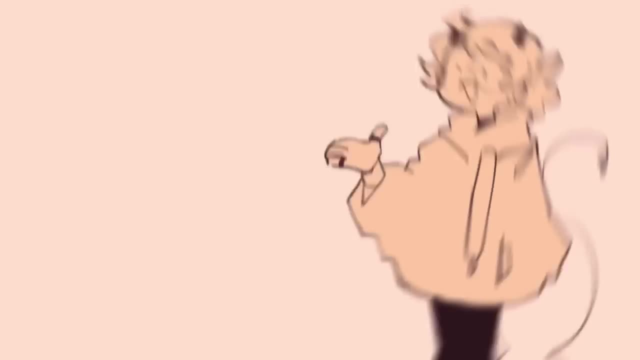 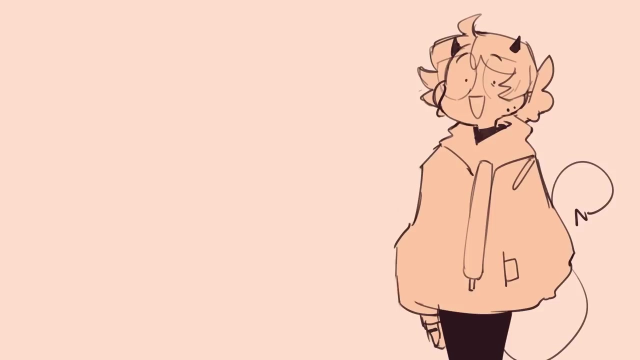 and have no focus point for the viewer's eyes to rest on. Though, if this is what you're going for, 100% go for it. Art doesn't need to have a set of rules. this is just what I like to think about. 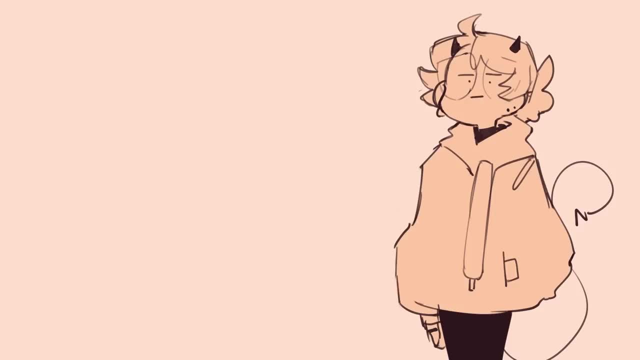 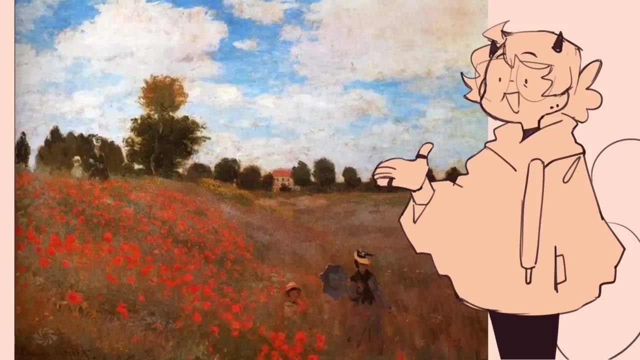 when I'm picking colours. Now this doesn't mean that highly saturated colours can't be used well in pieces. Highly saturated colours against desaturated colours can be used for contrast or to draw attention to specific colours, details or objects in the piece. 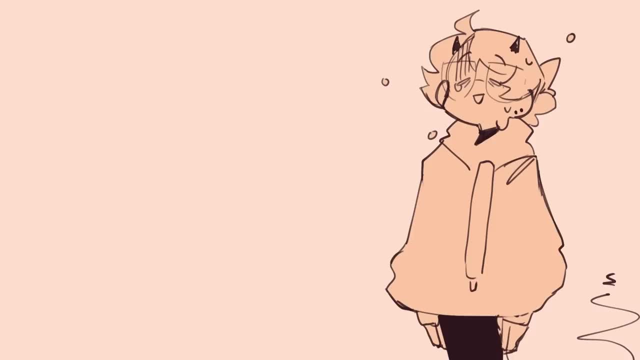 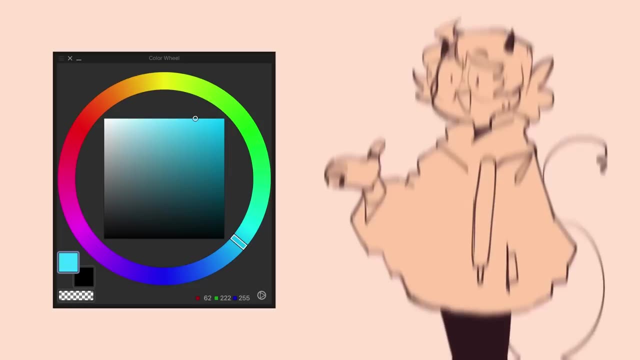 And I've seen a lot of people use highly saturated colours in their pieces and it looks very nice. Colour harmony is the colours that go well together. This can make a viewer look or feel a certain way. The colour wheel can be used to find colour harmonies, For example, yellow, orange. 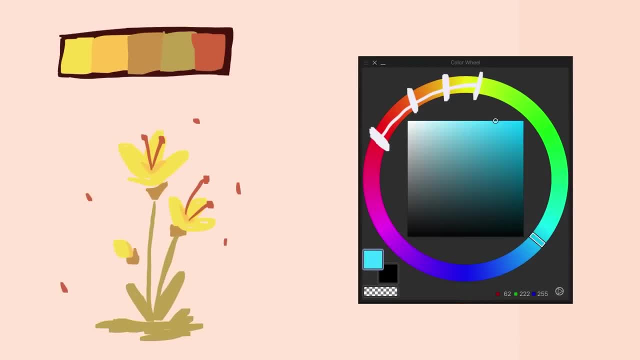 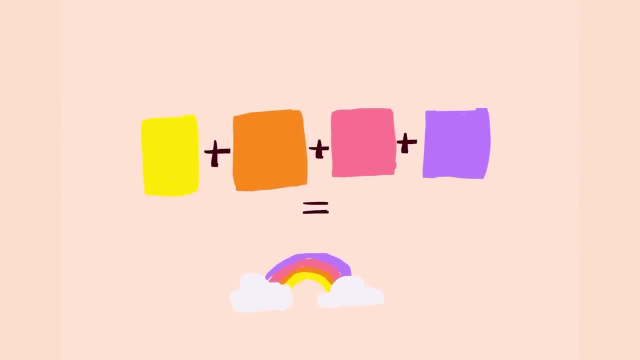 and red are colours that are really good together because they lie next to each other on the colour wheel. By using the layout of the colour wheel, picking colours that are pleasing or bold is easier by using the rules of colour combination, colour schemes or colour palettes, even if you 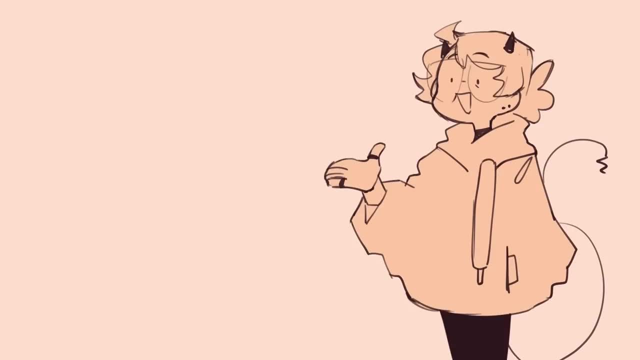 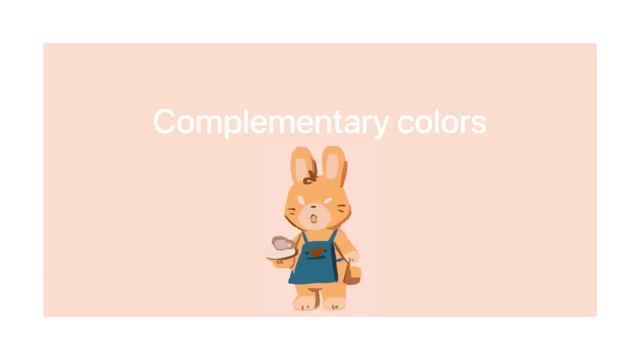 don't have a colour palette. Here are some colour combinations or colour schemes that look good together. I'll show you this by using the colour wheel, and I'll also show you where the colours can be located. First one is complementary colours. This is probably the one of the most popular. 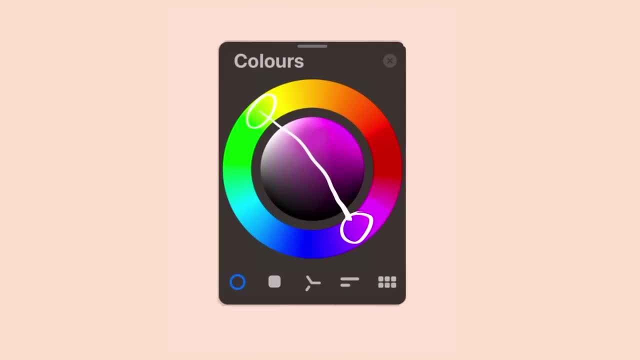 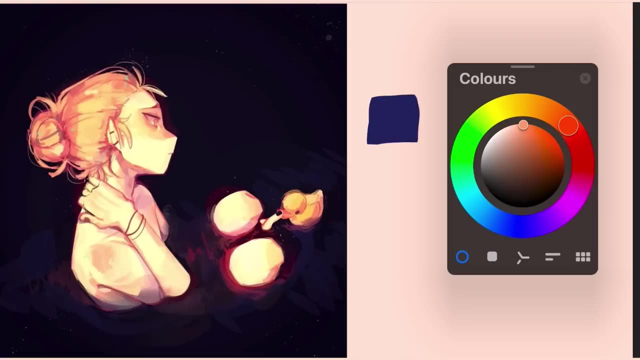 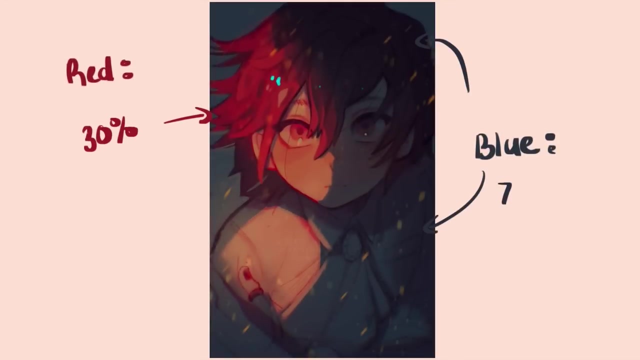 It's the use of two colours opposite to each other on the colour wheel, like red and green or purple and orange. Using complementary colours can give the art work high contrast and can be very vibrant and prominent. When you use the colour palette, don't use the colours equally, like 50-50.. Have one colour. 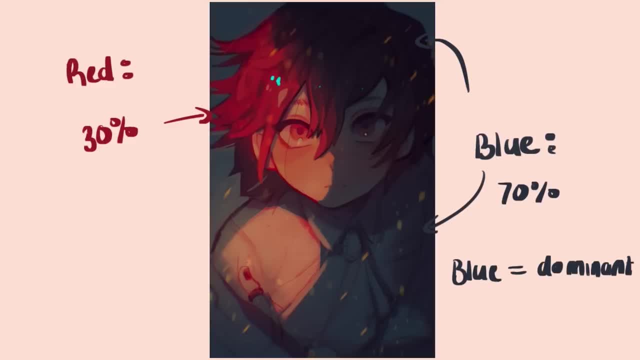 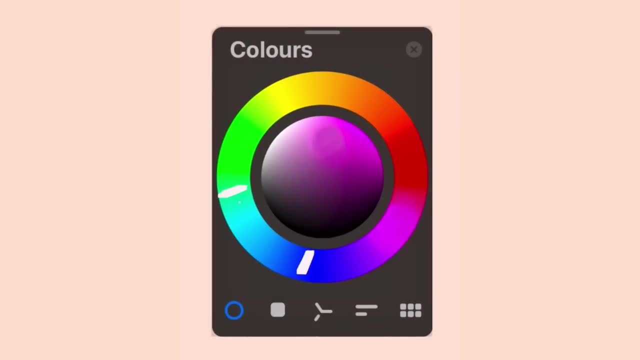 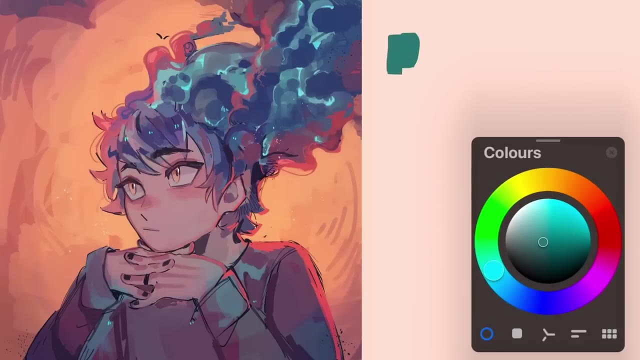 be dominant and the other be used as a highlight. Next is split complementary colour scheme. Similar to the complementary colour scheme, this one uses two colours that are close to each other on the colour wheel and then one colour on the opposite side. I make use of 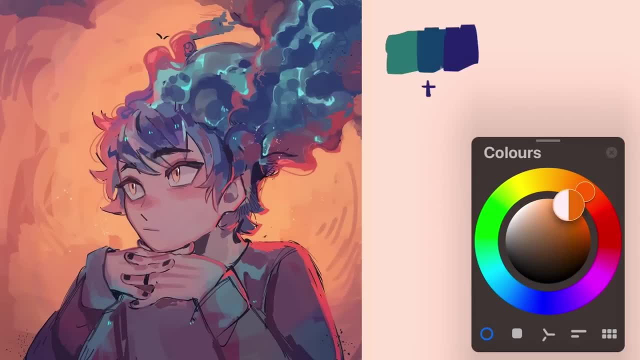 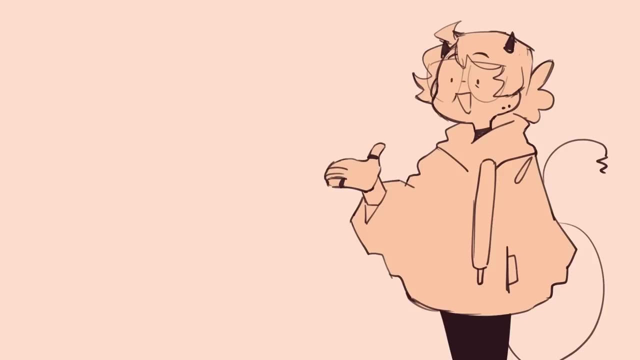 this one the most, since I love the deep contrast that the opposite colour can bring and still be very easy on the eye. because of the colours that are next to each other that create harmony, Following this one is my two most favourite harmonies to use. 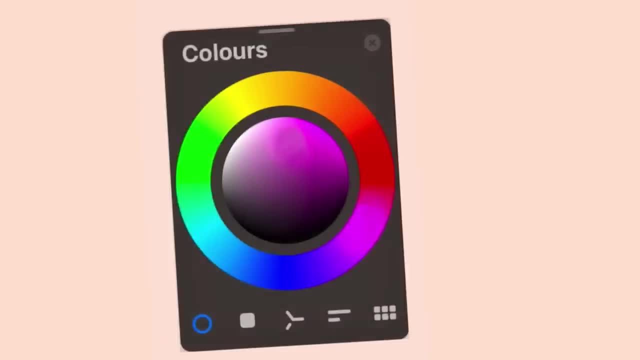 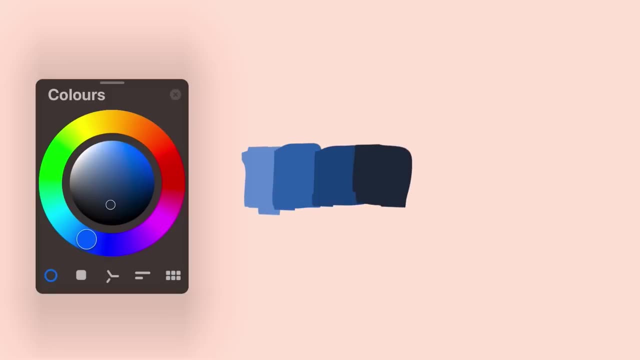 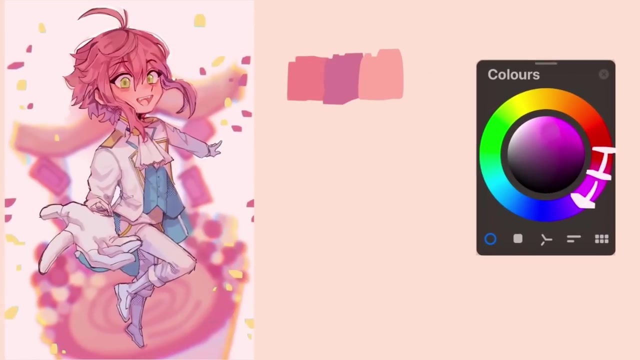 Monochromatic and analogous colour schemes. Both of these use tones and tints and values all in one or two colour hues. Monochromatic uses one hue and analogous makes use of more hues that are next to each other in the colour wheel. They create a peaceful and comfortable mood, since the colours are related to each other. 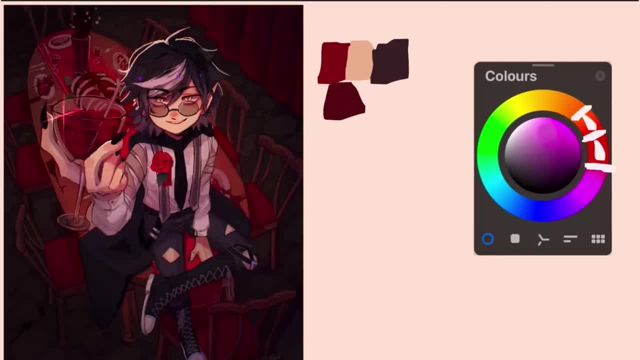 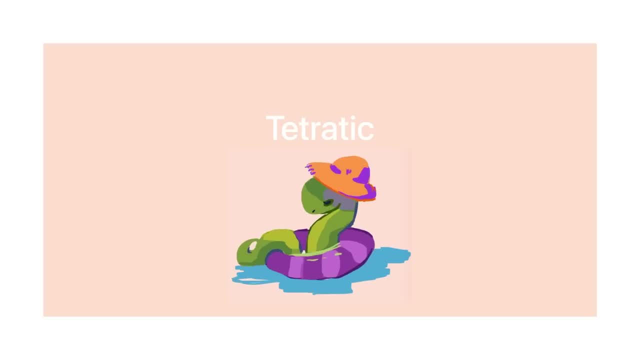 or next to each other on the colour wheel. Creating an atmosphere with these two schemes is a lot of fun once you learn the meaning of colour, which I'll touch on later in the video. Next is tetratic. This is choosing two pairs of complementary colours, similar to the last but with an extra. 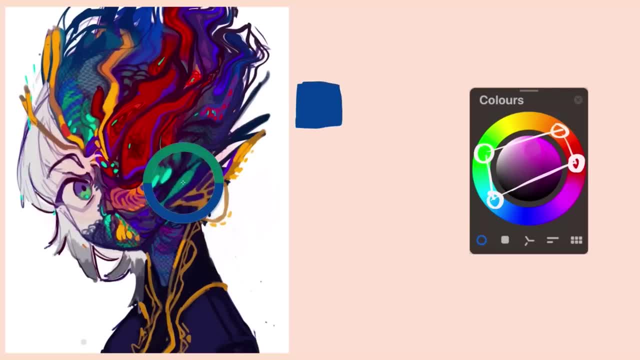 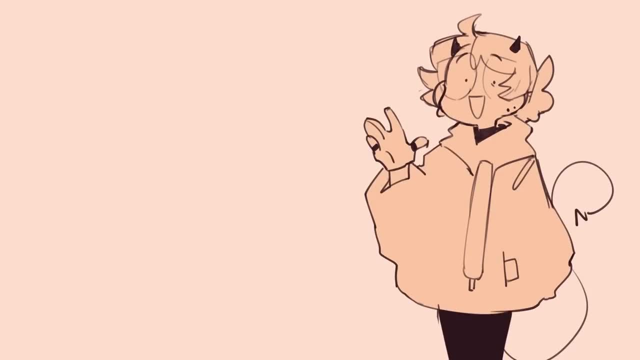 pair of hues added. This can create a pleasing set of colours, though it's harder to pull off. It's not a colour palette I use personally. Colours also have feelings, moods and vibes with them that will help communicate what atmosphere you're trying to convey in your art. 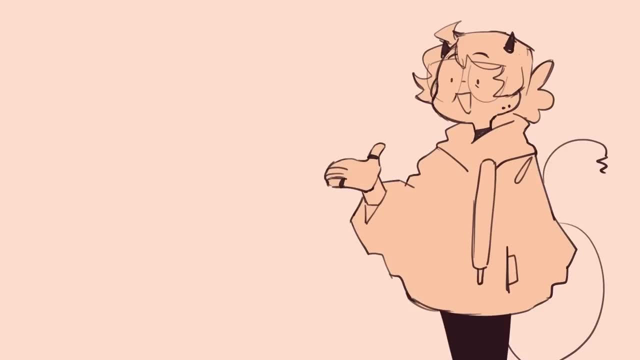 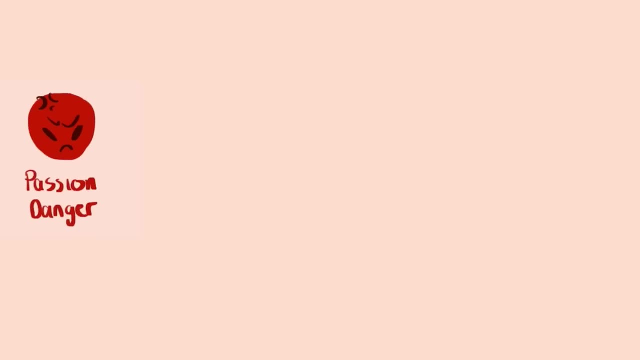 It's as simple as warmer colours will go with warmer and more aggressive emotions, while colder colours go with more cold and calmer and sad emotions. Here's a few examples: Like red is associated with passion and danger, orange is associated with energy and creativity. 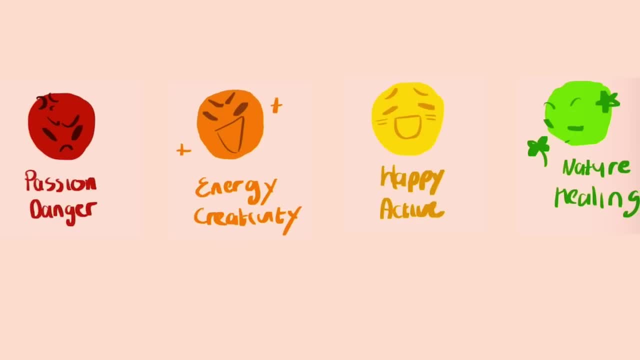 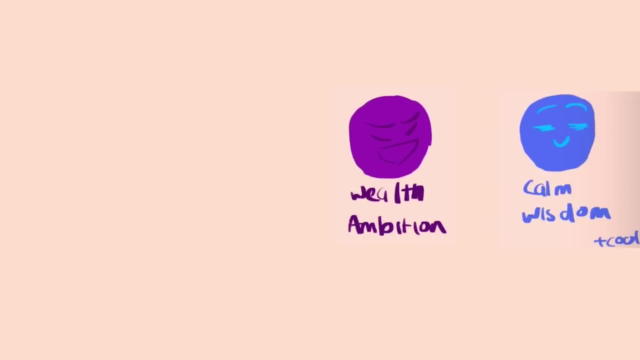 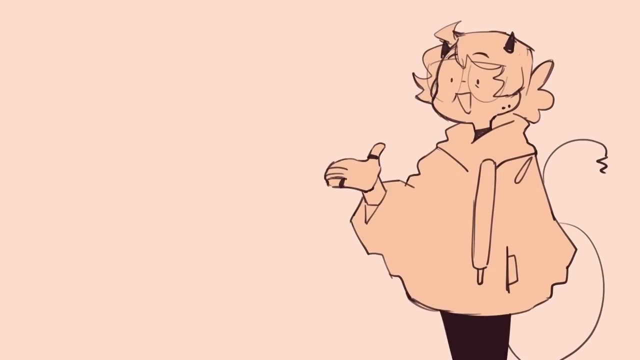 yellow is associated with happy and active. green is associated with nature and healing. blue is associated with calm and wisdom. purple is associated with wealth and ambition, white is purity and peace, and black is death and power. Adding these colours according to what emotion you would like to bring to the piece will. 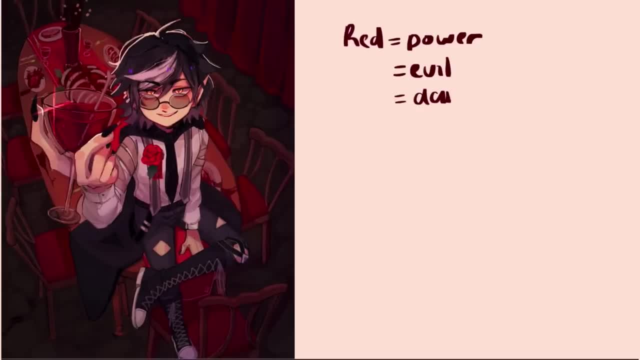 help convey atmosphere. I like to use these colours in my art. I'll choose the analogous colour scheme and choose hues that fit the piece Like. if it's sad, I'll use more blues and purples, but if I want to add a bit more of 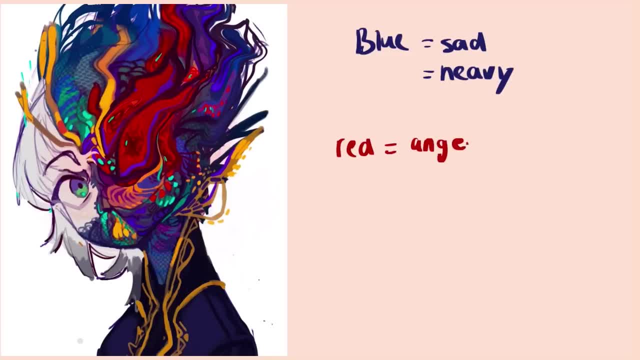 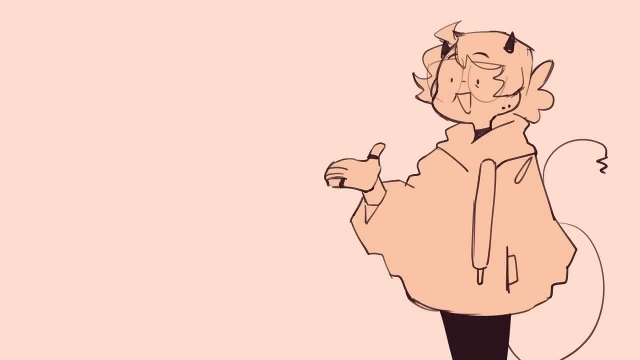 an angry element, I'll add a warmer tint of red. This will change the colour scheme from analogous to split complementary colour palette. Now we can go to the bit more trickier side of colour theory. Colour context is the effect of different values, saturation and hues. 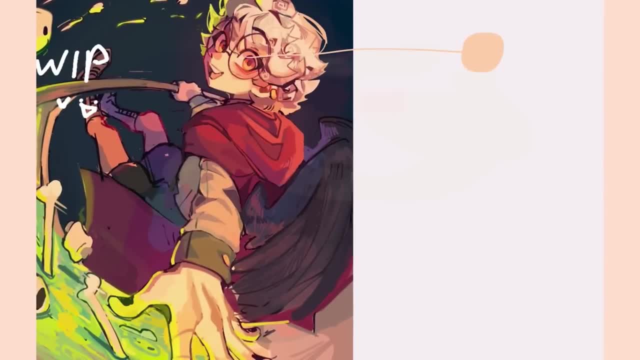 Like the warm or the coldness of a certain colour, can cause noticeable differences on how we perceive that colour. The way we see hues and values and saturations can be changed by surrounding hues, values and saturations. This is called simitunius contrast. 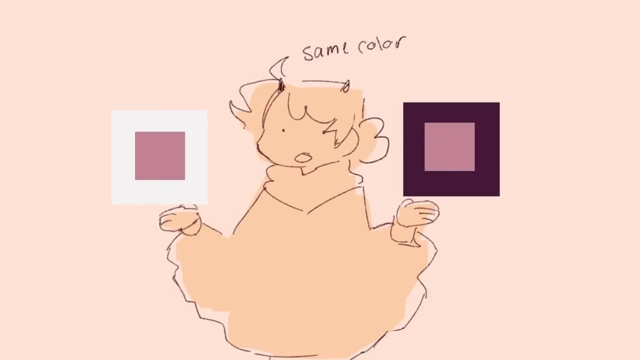 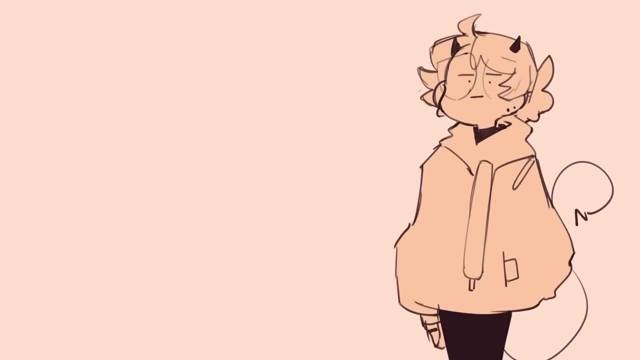 Here, for example, the colour in the middle is the same, but the background can make these colours appear a lot more different than what they actually are. Value is also affected by simitunius contrast. When a colour is placed in a dark background, it will appear lighter.